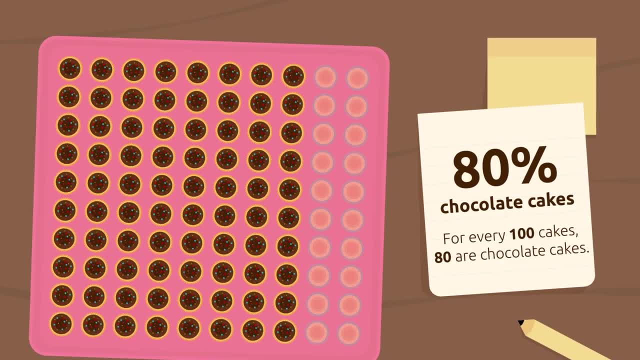 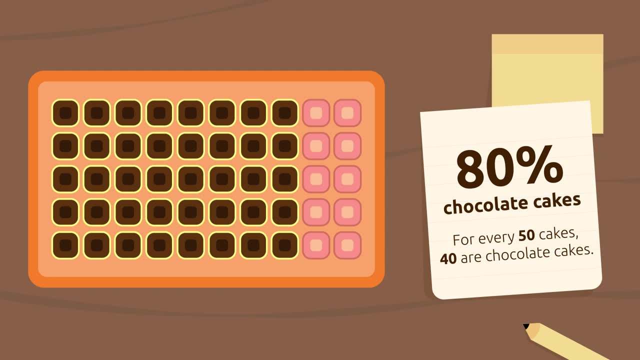 The number of elements doesn't have to be 100.. Let's look at 50 cakes, for example. 80 are chocolate cakes, 80 are chocolate cakes. 80% of them are chocolate cakes too. We use percentage to calculate all types of discount for products on sale. 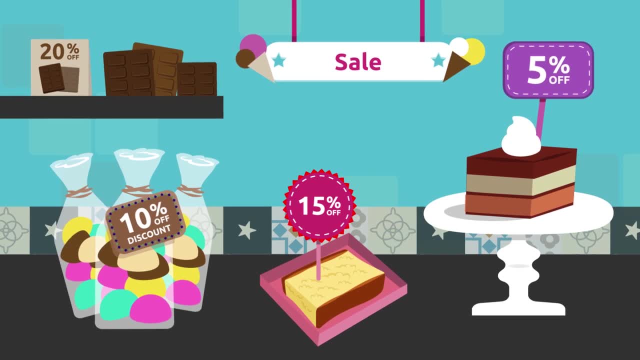 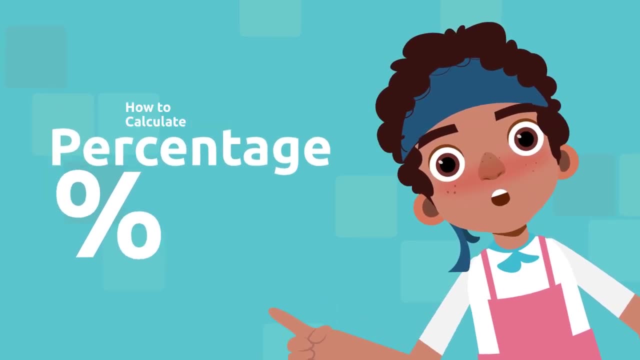 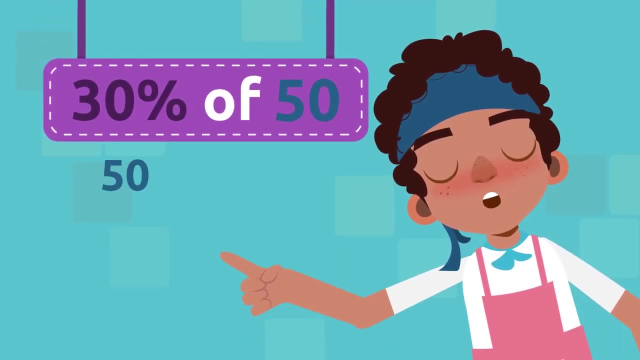 You can save a lot of money if you learn how to calculate percentage. Great, Now that we know what percentage means, let's find out how to calculate it. To calculate the percentage of a number, we multiply that number by the indicated percentage. 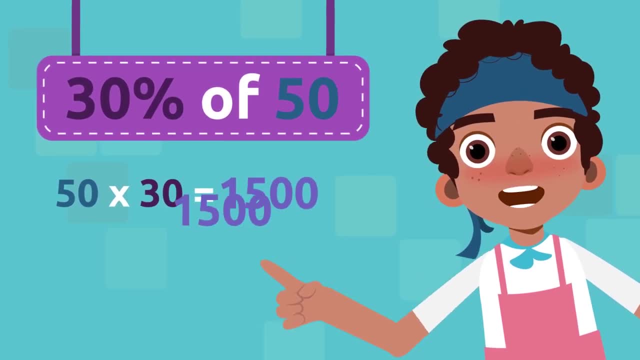 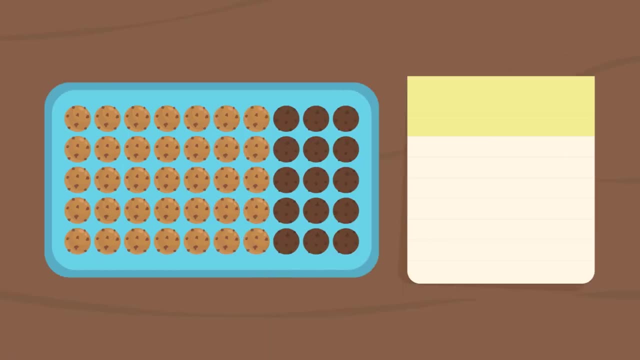 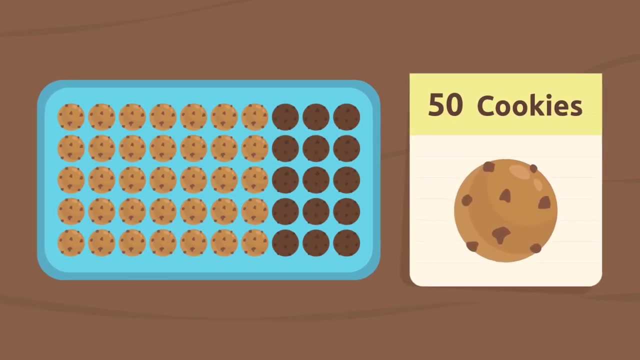 and divide by 100. We divide the percentage by 100.. Let's look at an example. Oopsie, What bad luck. I had to bake 50 cookies but got distracted explaining percentages and 30% of my cookies got burned. 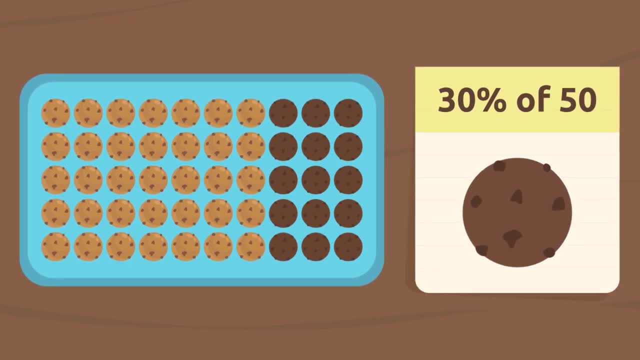 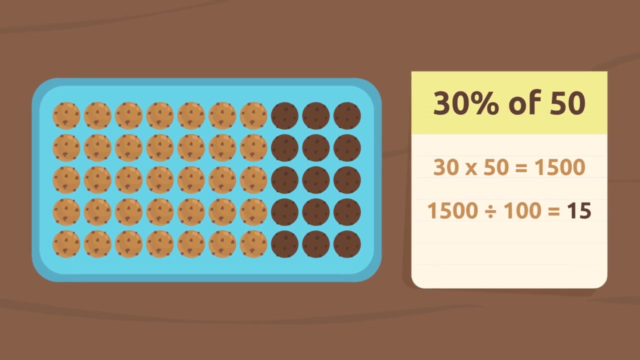 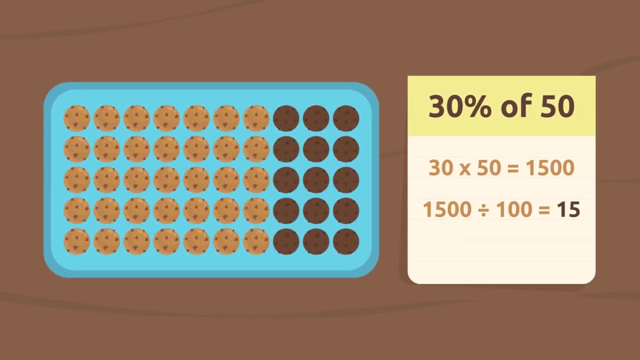 How many cookies actually got burned? To find out first, we should multiply 30 by 50. this equals 1500. then we divide this result by 100, which equals 15. so if 30% of my 50 cookies got burned, that means that I burned 15 cookies, did you? 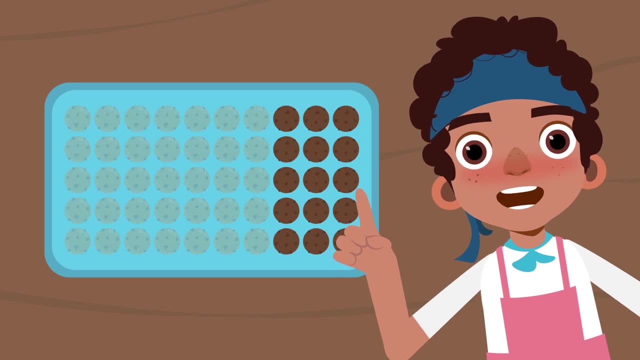 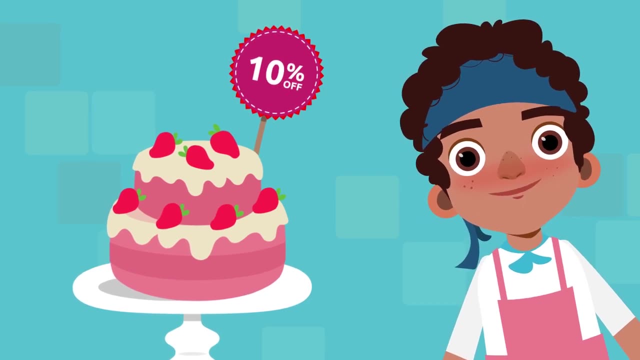 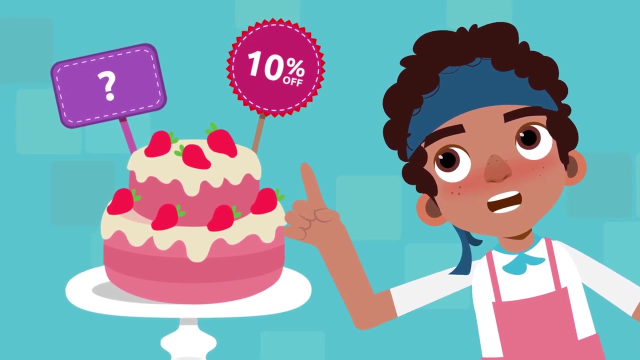 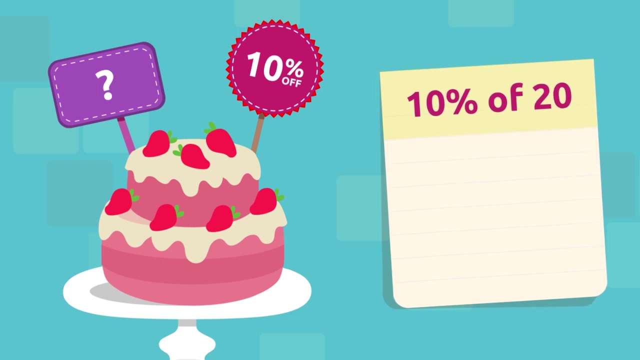 understand that. let's try with another example. just for today, the strawberry cakes have a 10% discount. their original price is $20. how much would each strawberry cake cost after the 10% discount? well, we just have to find 10% of 20. are you ready? I'm going to give you a few seconds to calculate that. 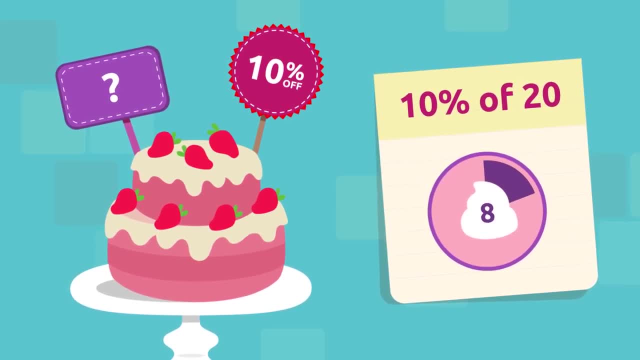 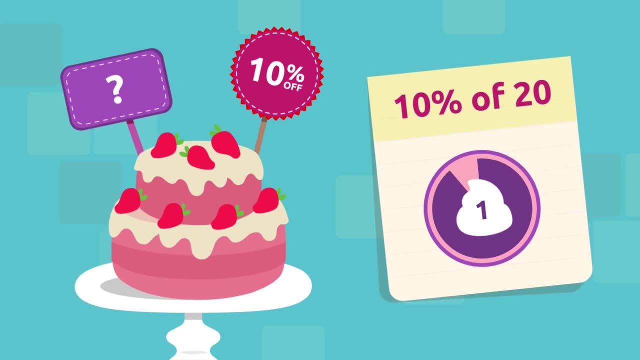 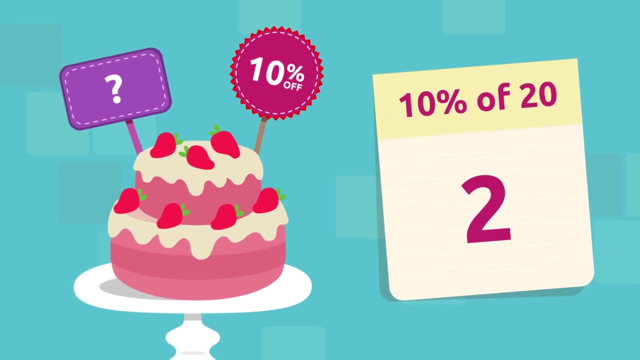 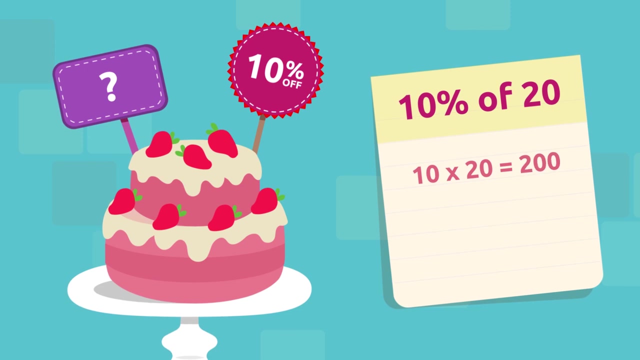 do you have the answer? 10% of 20 is. do you got that right? let's see: ten times twenty equals 200, and 200 divided by 100 equals 2. Okay, Rosister, what's 10 years old? then? we could multiply by 100 and divide that dinner into 2, we get 12, like whatever.